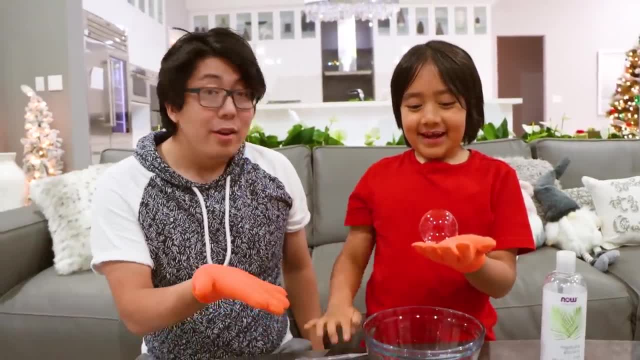 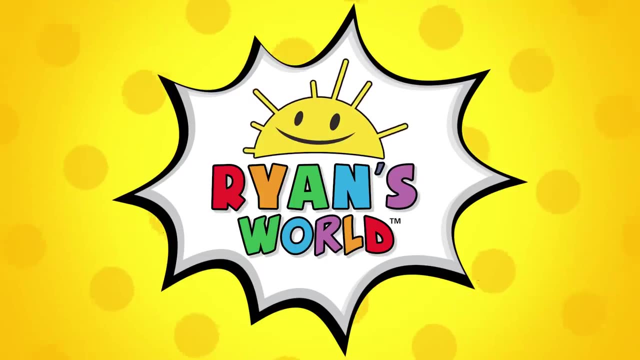 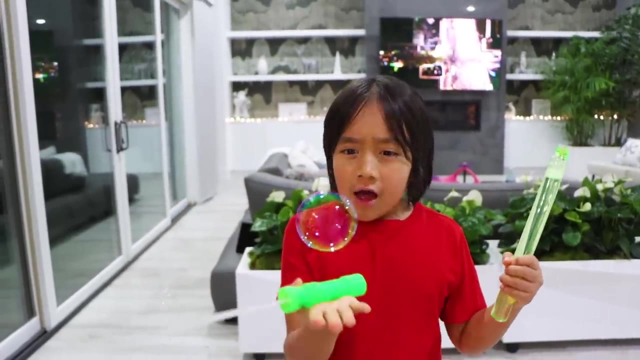 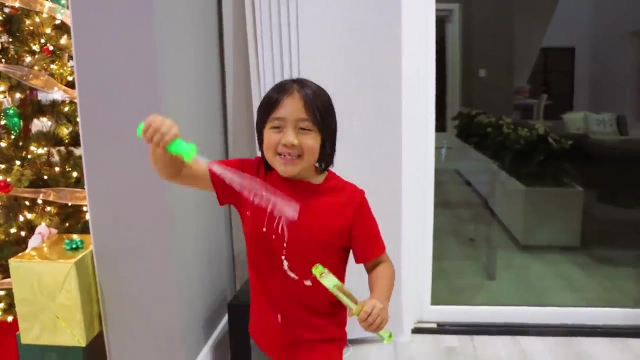 Whoa, Whoa, Stop popping. Whoa, It's bouncing. Welcome to Ryan's World. Hey guys, are you tired of bubbles that always pop Aww? Today I have a solution for you: Non-popping bubbles, Let's go. 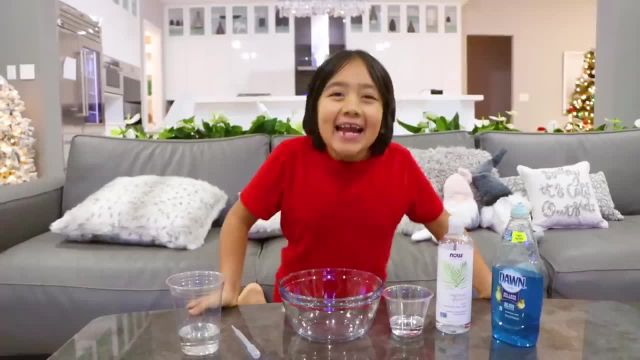 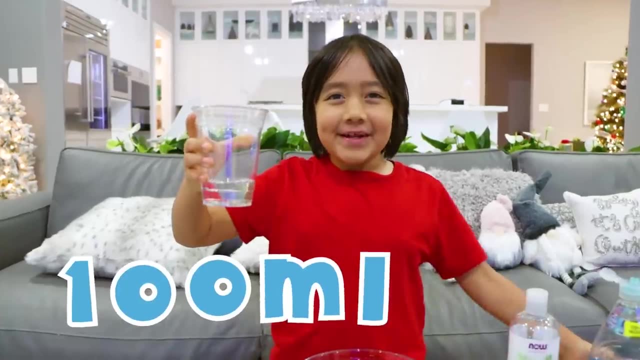 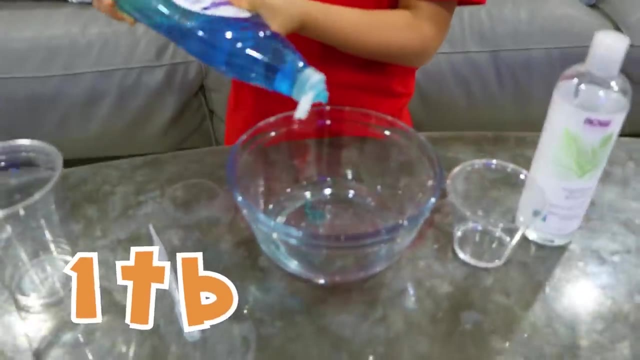 Hey guys, today we're going to make bubbles that don't pop, but always ask a parent for help. So first you need 100 milliliters of water and then 50 milliliters of glycerin, and a squirt or one tablespoon of Dawn soap. 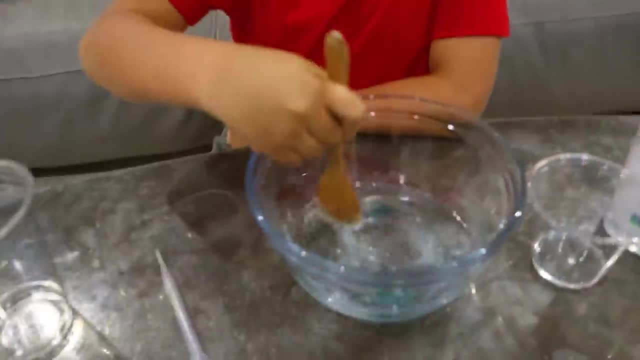 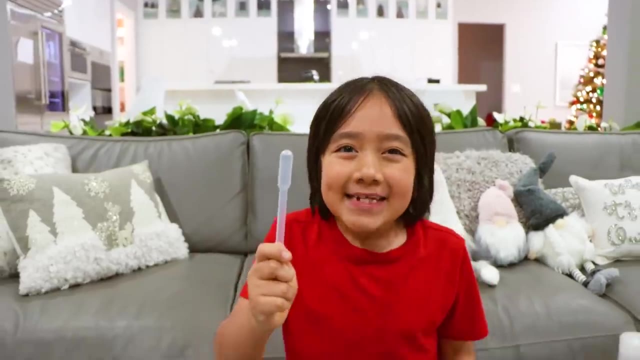 Next, let's agitate. or another word for mix. Next, get a pipette and cut it right here. I'm going to ask my daddy to help me. Hey, Ryan, Alright, so we're going to cut right here. Alright, I'm going to cut this for Ryan Boom. 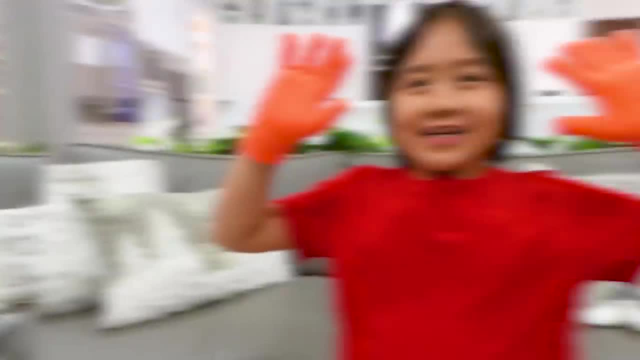 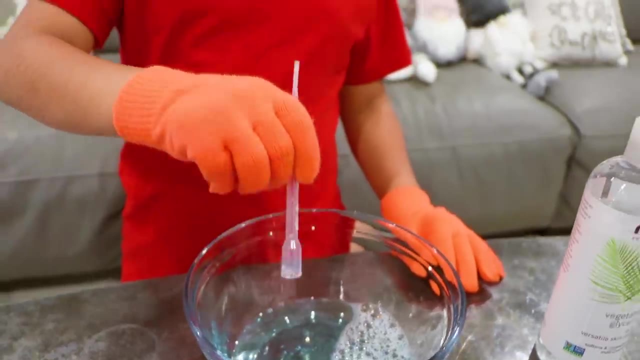 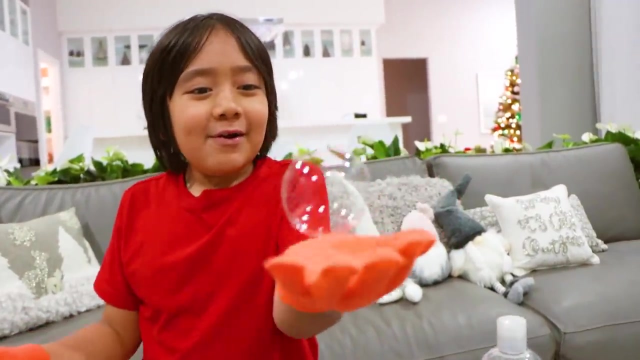 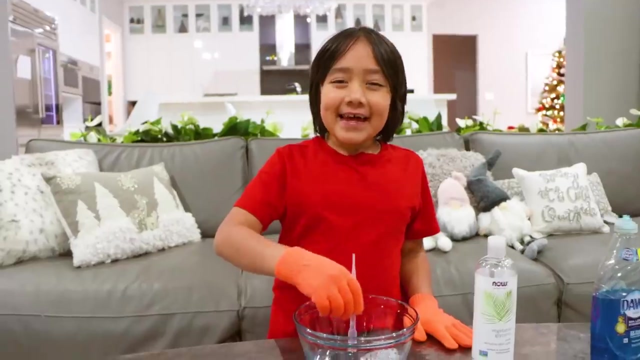 Is this what you wanted? Yeah, Next, you need some woolen gloves, and then you take the pipette, dip it in the water and glycerin, and then There you go. Whoa, Let's try that again. 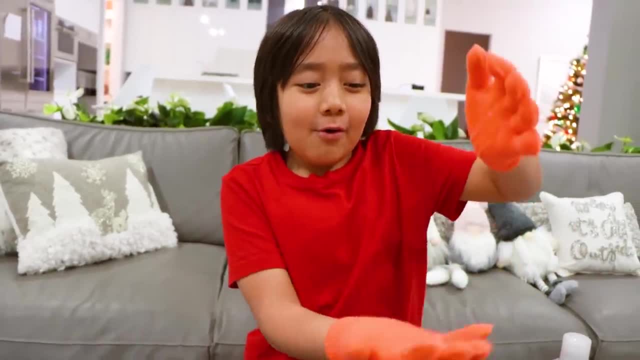 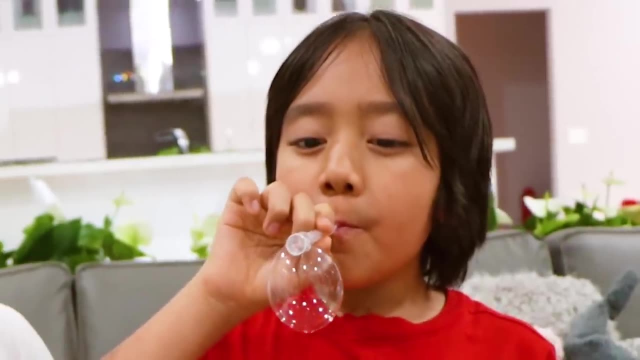 Okay, guys, we're going to see until it pops. Oh, It already popped. Now me and daddy are going to throw the bubbles to each other until it pops. Whoa, Whoa, Okay, Stop popping. Whoa, It's bouncing. 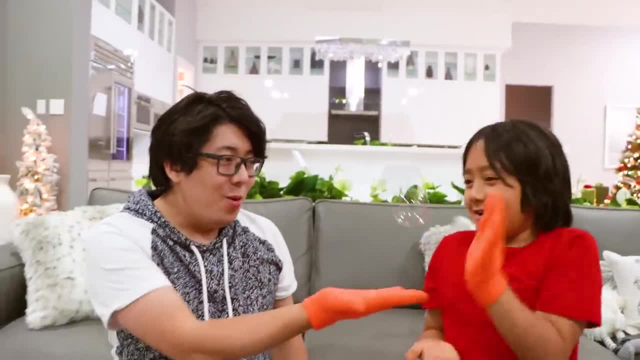 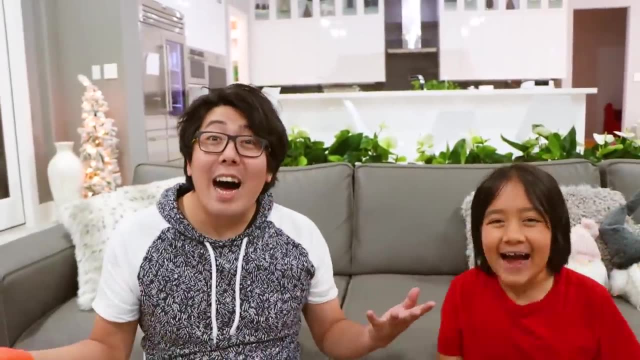 Yeah, Whoa, Whoa, Whoa, Whoa, Whoa. Now I almost tried my real one. Yeah, make sure you use your glove. Whoa Whoa Here. Whoa What I popped, I popped. 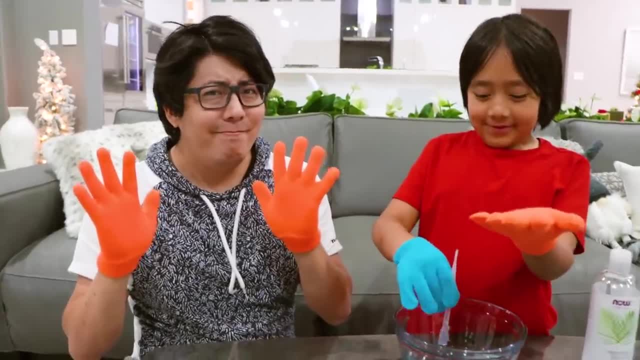 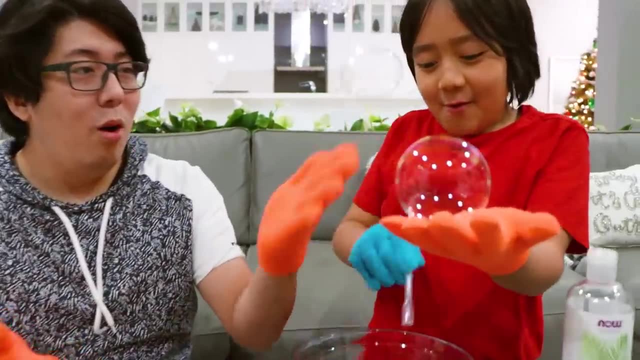 Okay, guys, now I'm going to make a bunch of bubbles and I'm going to see how much me and daddy can hold. We're going to break the world record. Whoa, Whoa, Whoa, Whoa, Whoa. 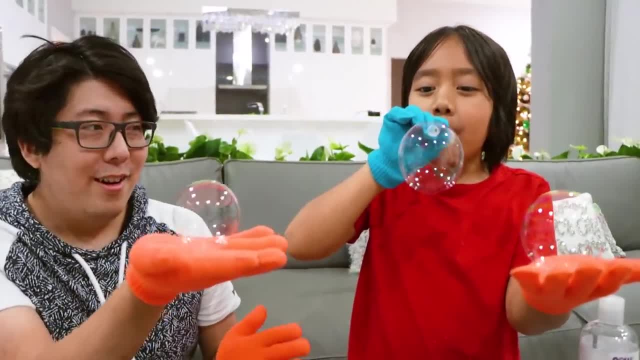 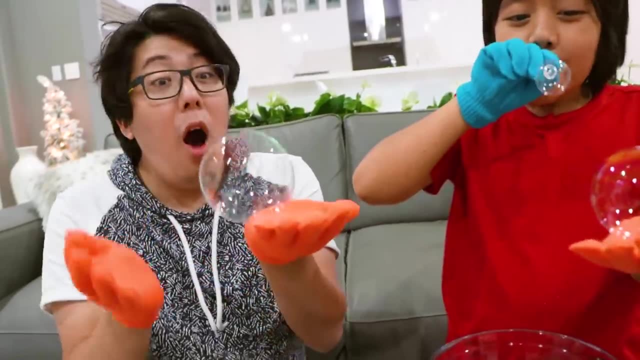 Whoa, Whoa, Come here. Whoa Ryan, That's huge. It bounced on your tummy. It bounced on my tummy. Can I put it together? Oh, Oh, Oh, Did you guys see? It became one.